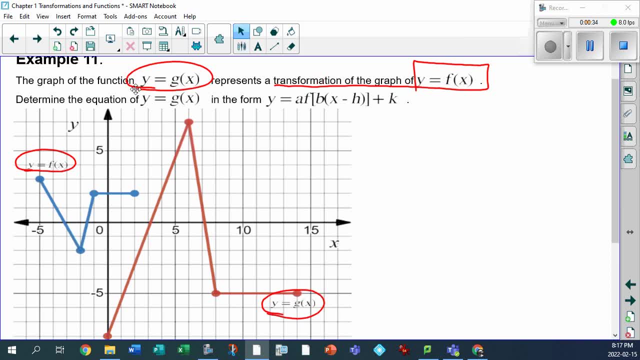 well, how do you figure out what's being done to it? Real simple. Read the rest of the question. The rest of the question says: determine the equation in this form. Well, that form tells you everything, doesn't it? The a, the b, the h and the k tell you all you need to know about. 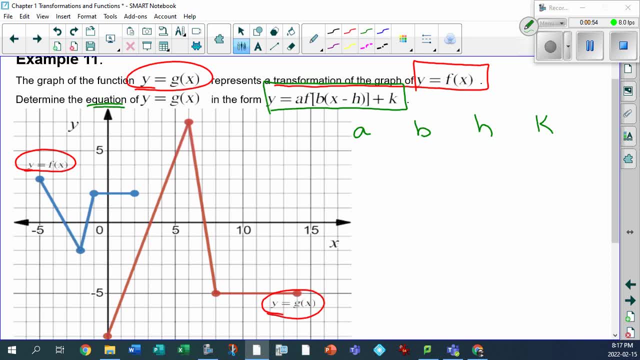 every single transformation that happens to this graph. Ah, cool. Now, so the whole point of this: if you figure out the a, b, h and k, you can figure out this beautiful transformation and put it right there and give me this new beautiful, transformed. 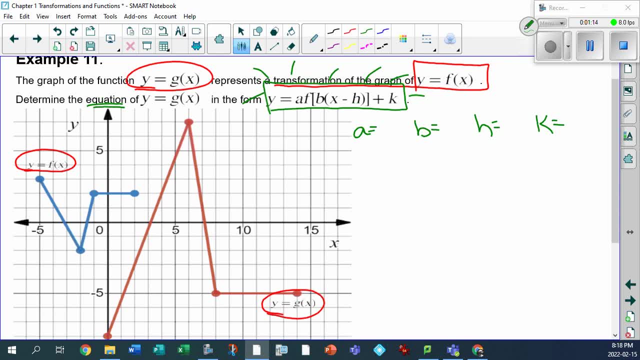 equation, Great. So let's do this Awesome. First things first. before you start making any calculations, take a look at this thing and see what kind of neat things have happened to it. Check this out. For example, graph kind of goes like this, doesn't it? Look at the new graph. Look at the g of x graph, If you. 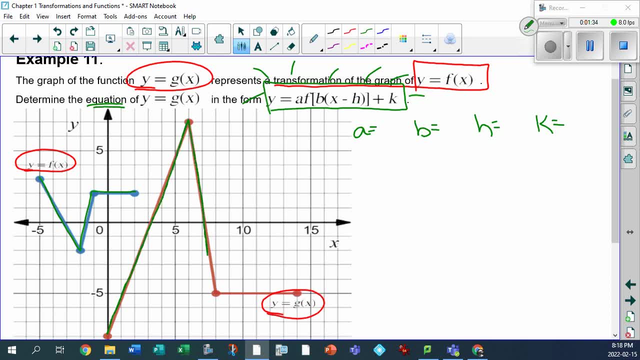 look at the g of x graph. huh, interesting thing happened. Look at this. This vertex looks like it's been. yep, the vertex has been flipped. It has been reflected over guess who. It's reflected over the x-axis, which guess what Means it's a vertical reflection. 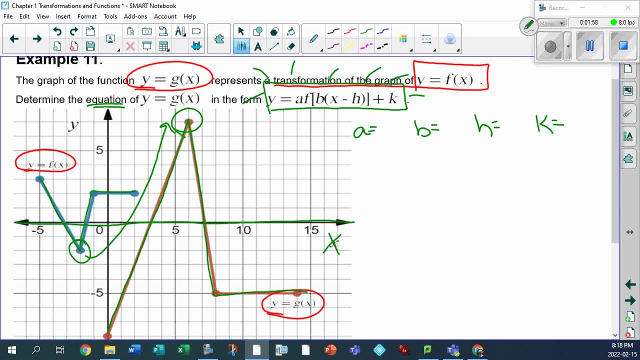 Now, do you remember? in a vertical reflection, is it a, b, h or k? It's your a value. Of course, to do a vertical reflection over the x-axis means that the a value has to be a negative. You see it Pretty cool, hey, Now here's the other thing I want you to look at. Look at the. 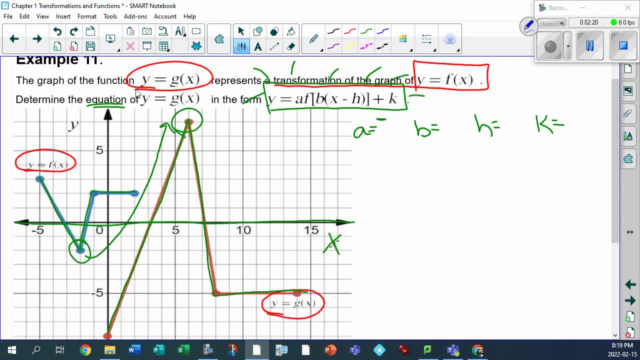 rest of this graph. Is there a horizontal reflection on this thing? Well, I don't know. Look at the stem. There's a little stem here, but look at this stem. Isn't this stem in the same general direction? So guess what? No horizontal reflection. This, in fact, is a positive Yay, Great, Now that. 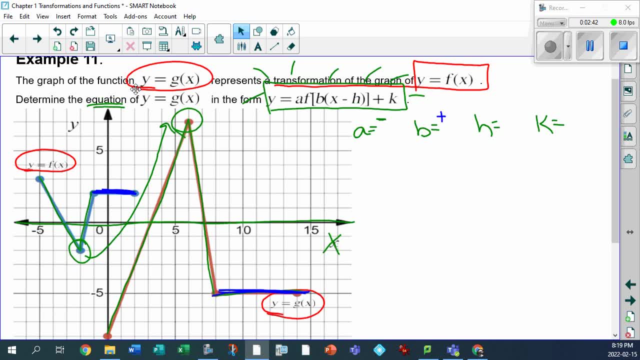 you've made all these observations, let's go out and find the actual values. So it's really good at first to look everything over to see if there's something that is absolutely obvious. Well, to me, that wonderful reflection, it was absolutely obvious, and now we know that we have to have this negative sign here in front of. 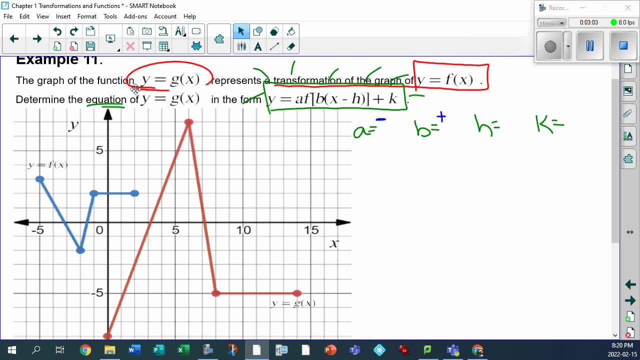 the a. Okay, great, So enough talk, Let's go out and figure out these values. Well, isn't a the vertical? Let's figure out the vertical. then Take a look at our original graph. Let's look at. 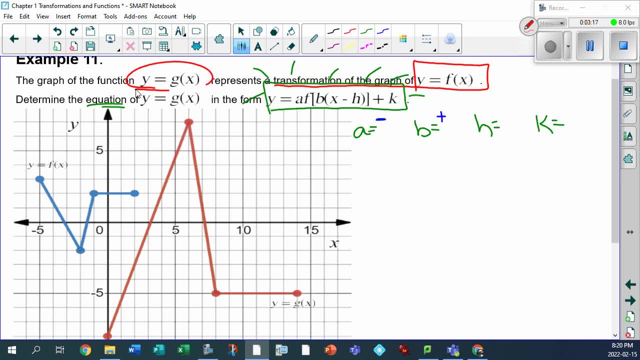 the height of this original graph, From the top here all the way down to the bottom. Check it out. There's the top to the bottom. Count it One, two, three, four, five. Oh, looks like five. Okay, Now compare the transformed graph: Okay. 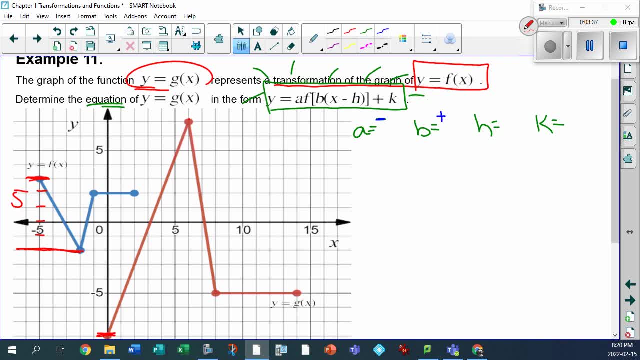 From top to bottom. Well, there's the bottom, There's the top, So count, Okay. One, two, three, four, five, six, seven, eight, nine, ten, eleven, twelve, thirteen, fourteen, fifteen- This guy's- 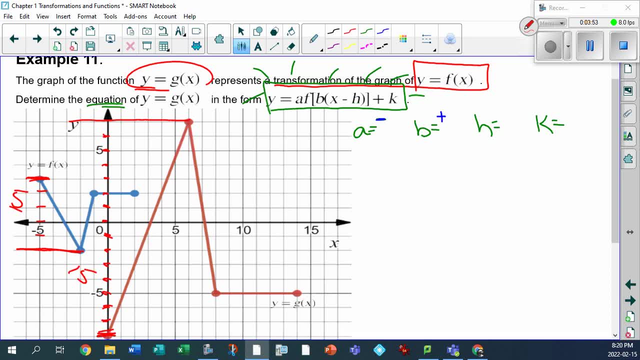 actually fifteen units compared to this guy five units Now. do you remember grade eight math? Yeah, I know what you're probably saying. Grade eight math was the best three years of my life. Okay, Good for you. There was a wonderful thing called ratios in that, and you 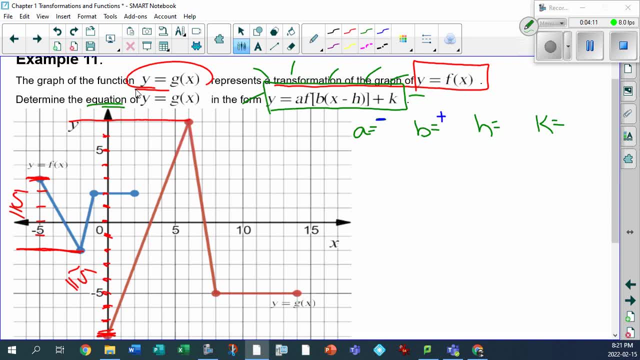 looked at scale factors in grade eight math. So how did you do the scale factors? You looked right on the graph. You saw that this was five, this was fifteen and you know to go from five to fifteen was a multiple of three. There's your scale factor. 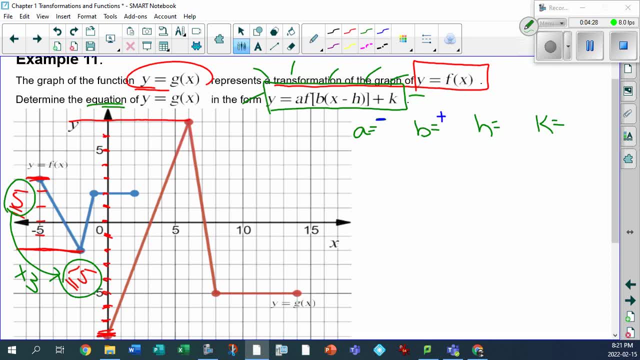 Oh, my goodness, And that's not just any scale factor. That is your vertical scale factor, And there's the three right there Along with the flip, you now have the A value Wild. hey, That's just awesome. Okay, So let's do the same thing to the horizontal, So I'm not going to have to look at. 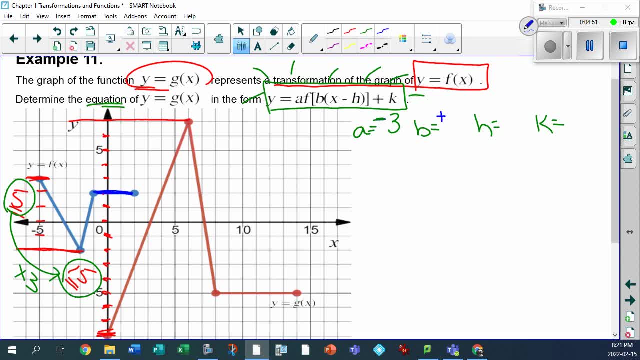 the entire graph. I'm just going to look at a portion of the graph. You can look at the entire thing if you wanted to. But if you're not going to look at the entire graph, you can look at the whole graph. So if you magnify, or I should say you stretch a portion of the graph, you stretch. 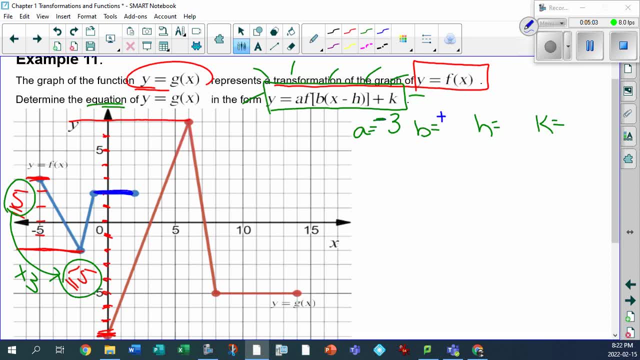 the whole graph. So whatever happens to a little piece of it right, will happen to the entire graph. So the entire graph gets stretched the same amount. So I'm going to look at this little stem here, compare it to this stem right here, So I don't have to look at the entire graph if I want. 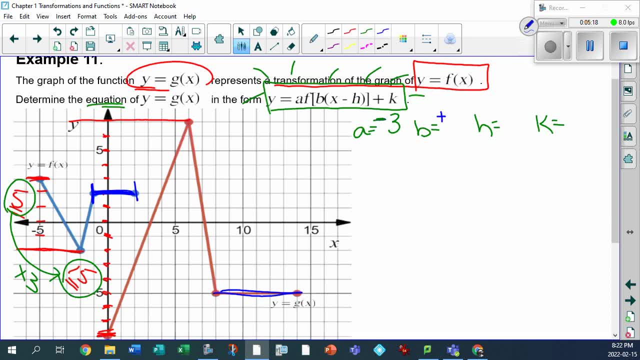 to Okay. So from here to here, count it: One, two, three, That is a distance of three. Okay, Compare this one. Look: One, two, three, four, five, six, That's a difference of six or a distance of six. Scale. 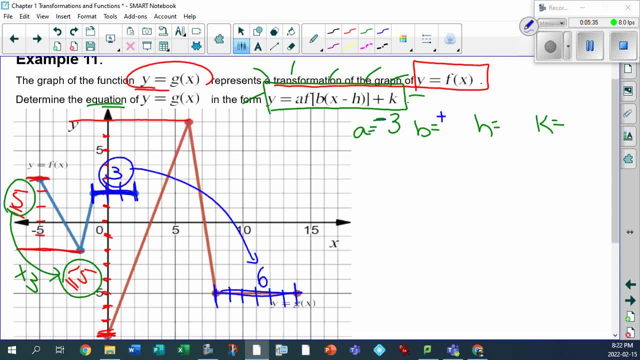 factor time: grade eight. How do you go from three to six? Yep, It's a scale factor times two. Oh, my goodness, Was it that easy? Almost Remember. this is the B, Don't get stung. Uh-uh. This is a scale factor of two, which means the B value is: 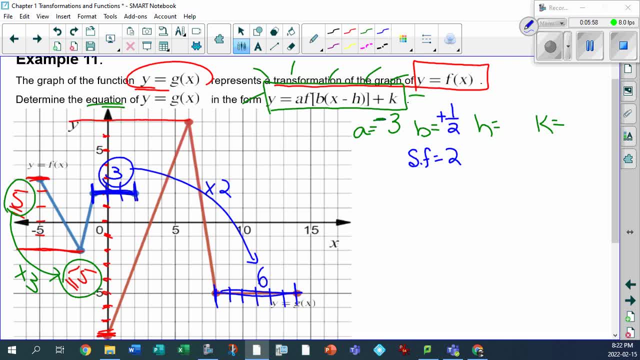 Yeah, you got it. It's a half. Ho-ho, You have to flip the B value, remember? Oh man, Yeah, Okay, So great. Look at this. We got half the problem done already. Oh, magnificent, Okay, So let's. 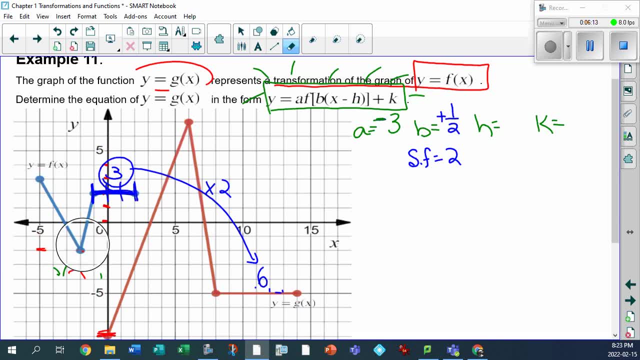 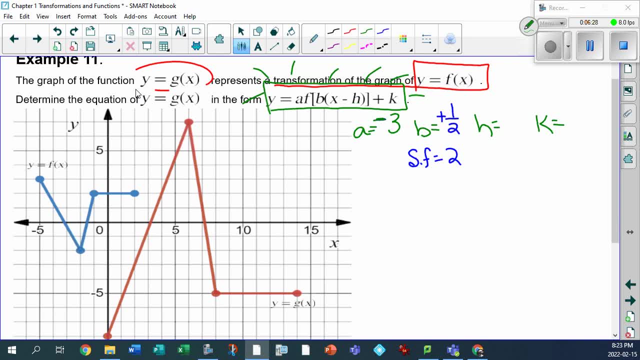 It's actually been put into this particular graph already. To find the H and K value, you got to do a little bit of work, But what kind of work do you have to do? You know what? I'm going to concentrate on one point and I'm going to see how we move that point. What point am I? 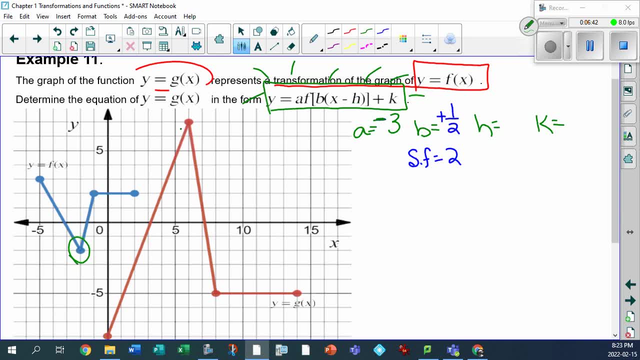 talking about The easiest point in the world. Look at the vertex. Look how that vertex just stands out, doesn't it? You can pick any point you want. I'm going to pick that beautiful vertex And I'm going to look at this original point 1, 2, that's negative. 2,. 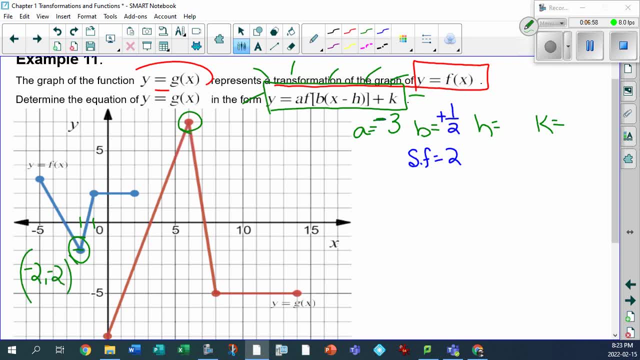 1, 2, that's also negative, 2.. There's my original point. Now I want to see how I got transformed that point to this vertex up here which is at: oh look, 5, 6.. That's going to be 6, comma 1, 2, 3, 4, 5, 6, 7, 6, 7.. 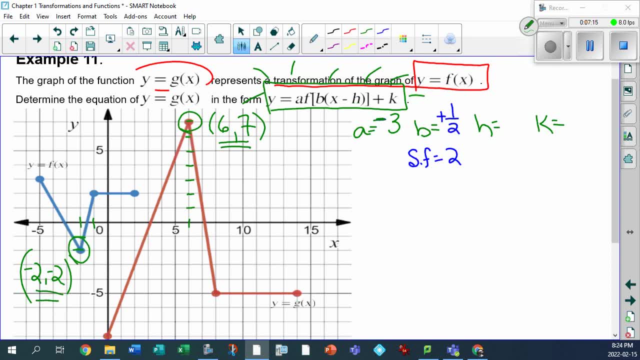 So this is my transformed point. This is my original point. Are you with me? Perfect, Now we are dealing with points. so that means guess what? Yep, we have to do a mapping. a mapping of point x, y to what? 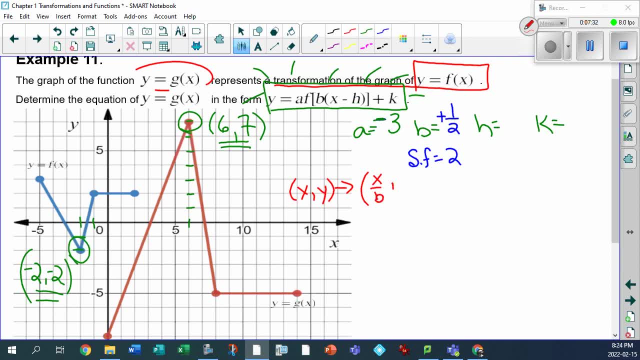 Well, you know and I know, that's x over b plus h, a, y plus k. Are you with me, You betcha? So look what we're going to do. We're going to take this point. We're going to go to here based on that mapping and based on uh-oh. 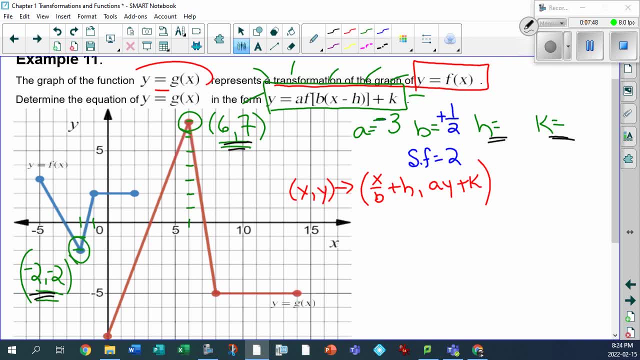 we still don't have the h and the k. Aw man, Okay, so think about it. We have the two points. We should be able to find the h and the k. Well, how? Let's put the a and b in there right now. 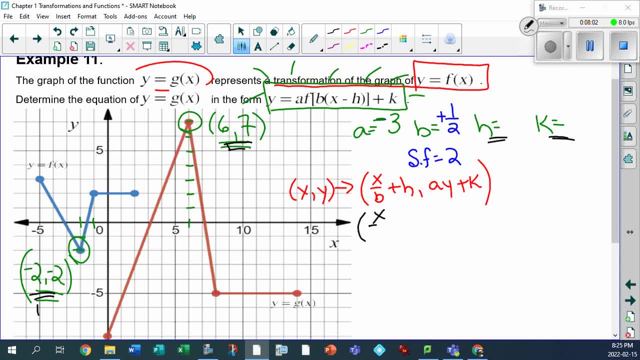 Let's see what happens. So this, of course, is going to be x over the b, the b being 1 half plus h, a, which is minus 3y plus k. Okay, beautiful, Excellent, Perfect. 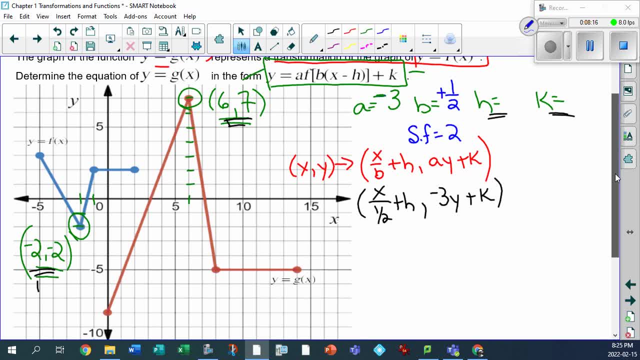 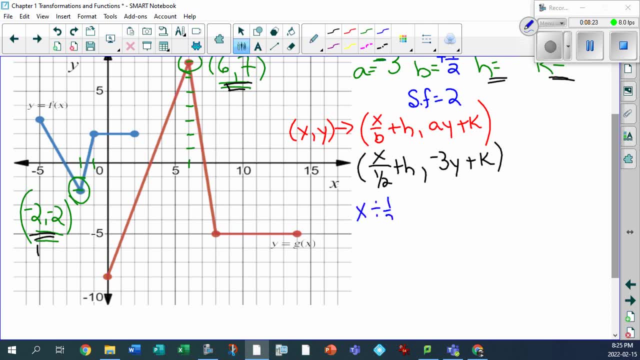 But I don't know about you. I certainly don't like that. x over a half, Do you? Nah? But think about what that means. That means x divided by a half, doesn't it? Which, if you remember your great seven fractions, that means x times the reciprocal. 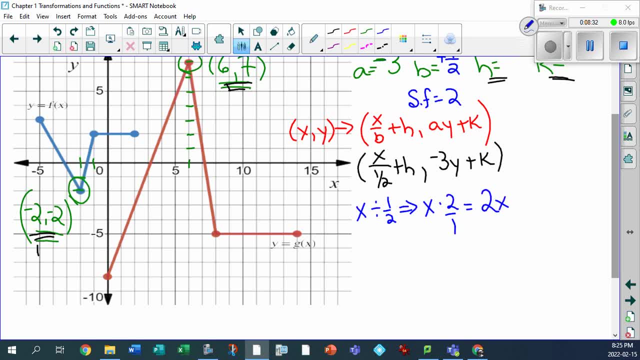 which is 2 over 1, which means 2x. Wait a second. Isn't that what we did? Wasn't this in fact 3 and this is 6?? If that was 3 and that was 6, the scale factor of this is times 2.. 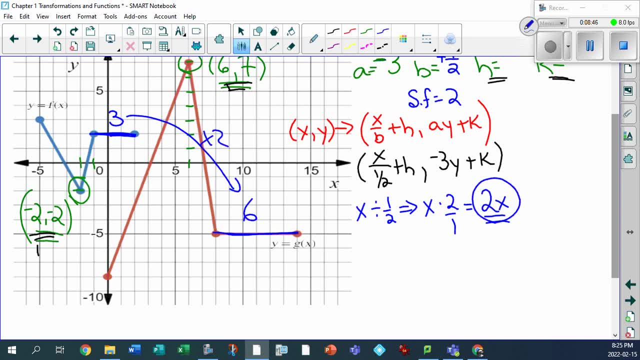 Well, that's what you were doing Every point times 2.. Doesn't that make sense? Certainly, So let's keep on going then. If that's 2x, watch what happens to this beautiful transformation here. This now becomes xy goes to. well, it's now 2x. 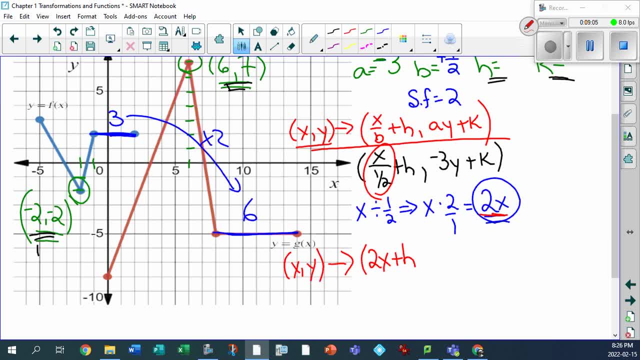 So this becomes 2x plus h, minus 3y plus k. Oh, you know what. We're so close, but you bet you just don't see it yet, do you? Let me show you how this works. The original point was minus 2x. 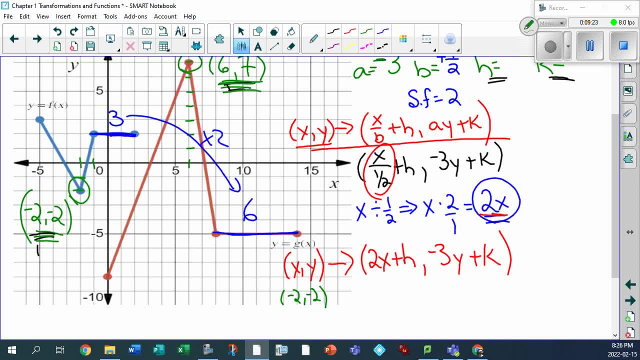 Minus 2.. The transformed point was 6 comma 7. So in other words, you had to use this equation here to get to that 6.. Take this minus 2 and get to that 6, right? Well, it's actually pretty easy from this point on. 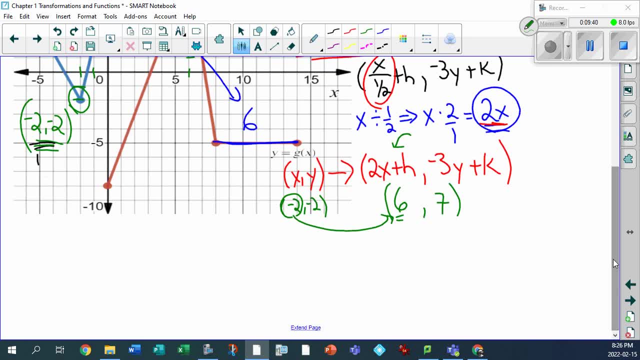 You probably don't see it yet, do you? Well, think about this. Is this not the equation to give me the transformed point? The transformed point being y prime Or, sorry, x prime equals to 2x plus h. Are you with me? 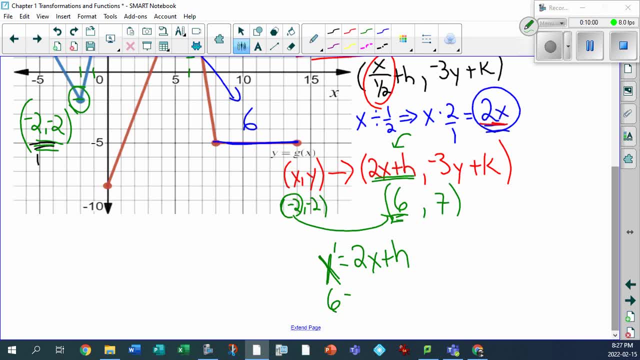 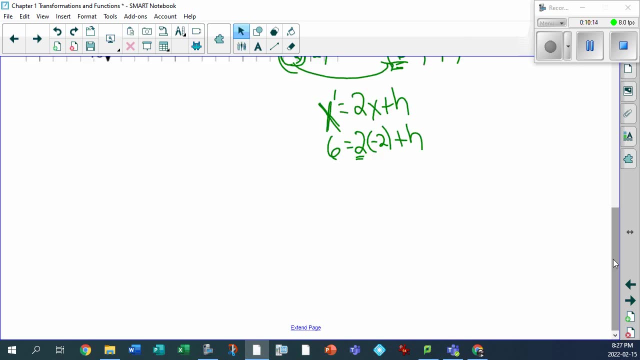 The transformed point 6, equals to the original point minus 2,, stretched by a factor of 2, plus some sort of horizontal translation. All we got to do now here is solve it. Oh, you're kidding, This is 6 equals to 2 times minus 2, which is minus 4.. 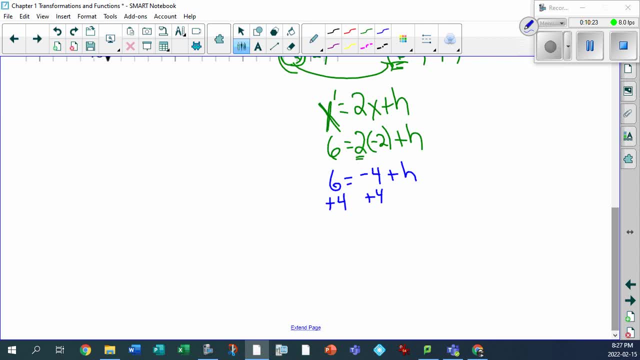 Plus h, add 4 to both sides. Oh my god, look what you got. h equals to 10.. There's your horizontal translation. Wow. So now all you have to do is go back to here and look what we've got. 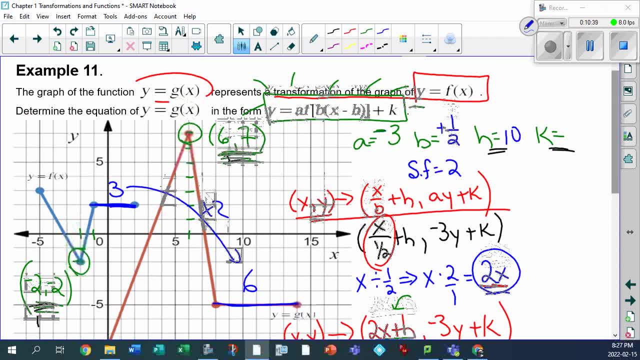 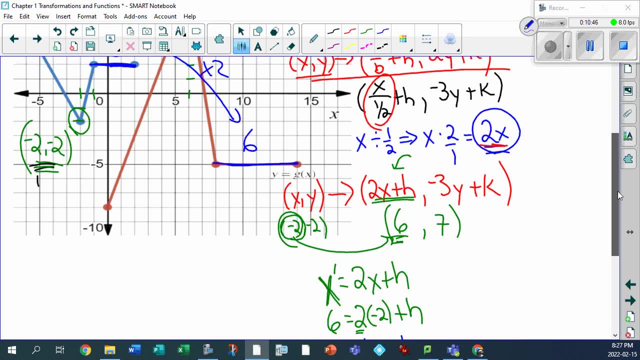 We've got the h to be 10.. Ha, All we got left is the k. Does the k work the same way? You betcha, Watch this. Let's go back to here. Remember what this meant. This was our y prime. 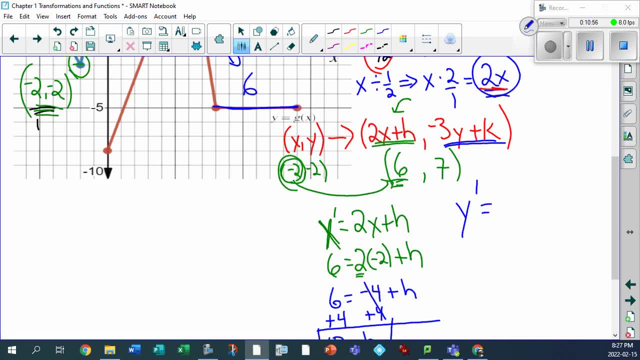 This is to find the image point. It follows that formula of minus 3 times the original y value plus k. All you got to do now is just substitute things in. What is y prime? Well, the y prime. oh, there it is. 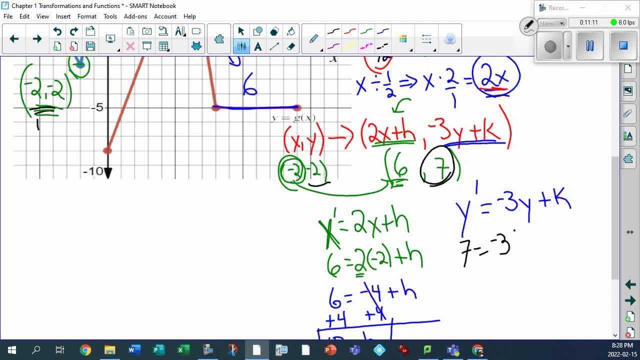 It's 7.. 7 equals to minus 3 times the original point, which is minus 2.. Beautiful Plus k. Minus 3 times minus 2 is positive 6.. So 7 equals to 6 plus k.